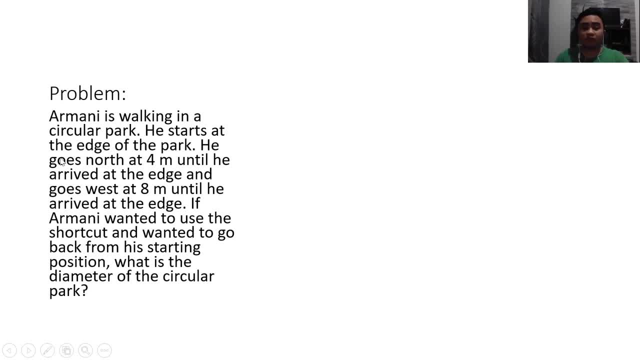 what is the diameter of the circular path? So the first thing that I'm going to do is to visualize the problem. So it says here that Armani is walking in a circular path. So the first thing that you need to do is to visualize the problem. So the first thing, 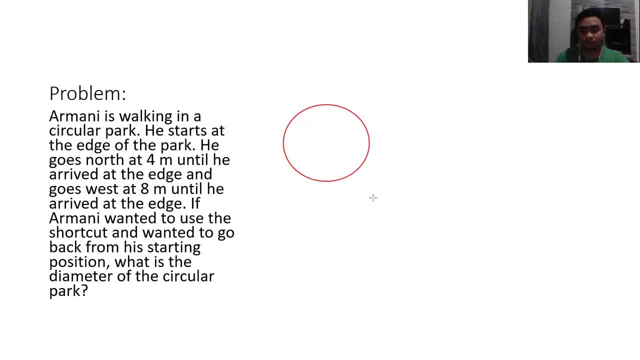 that you need to do is to draw a circle. So we have this one There, For example. that is our circle. It says here: he starts at the edge of the park. He goes north at 4 meters until he arrives at the edge and goes west at 8 meters. So that's what I'm going to read. 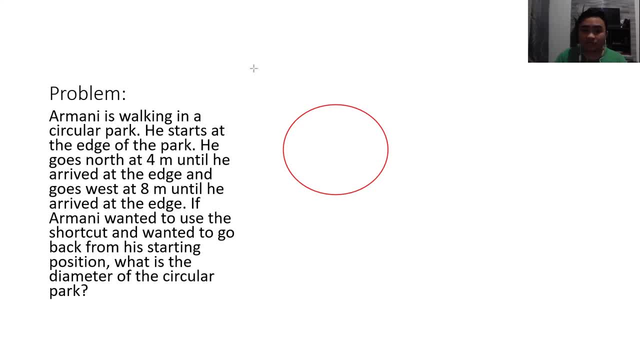 in this rubric so that it's easy for us to identify where we're going to draw. For example, we're going to draw a circle, So the first thing that I'm going to do is to visualize the problem. So, in this case, 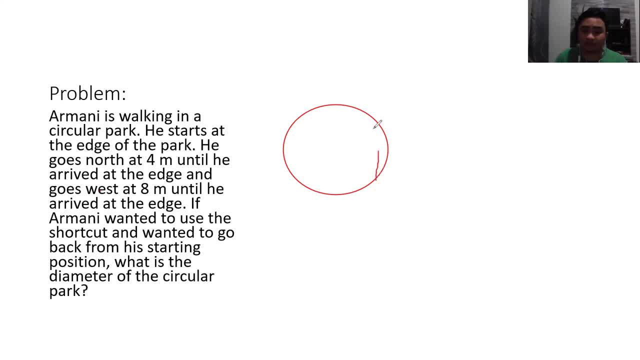 since Armani goes west. so this edge probably is this one. So I'm going to undo that. Let's say that he goes north at 4 meters. So let's say that he goes north at 4 meters. So let's okay. and then, 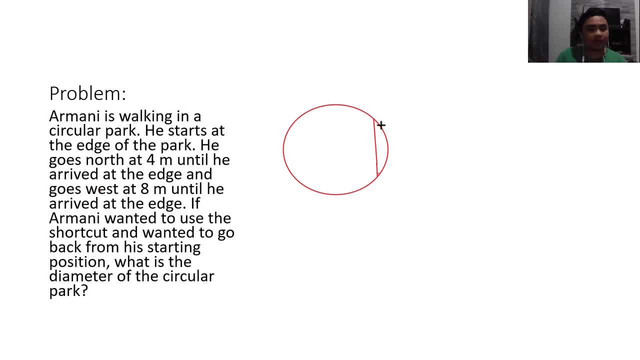 There. Next he goes west at 8 meters. So let's follow going west at 8 meters There. So until we arrive at the edge. if our money wanted to use the shortcut and wanted to go back from the starting position, what is the diameter of the circular part? 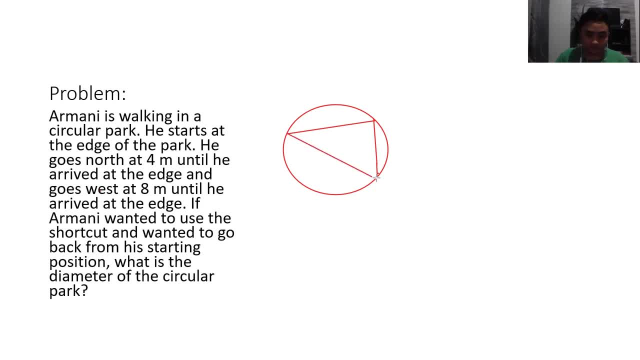 So we will use also this one. So, given Let's say, for example, that this circle is circle A There, And then these points are So, how are we going to solve that? So let us have: 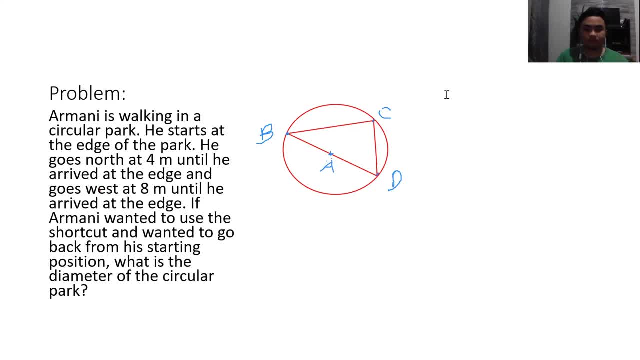 This one In circle A, let the given. So he goes north at 4 meters. So let's put here 4. And here is 8.. So let DC or let lines Line segment. DC is equal to 4.. 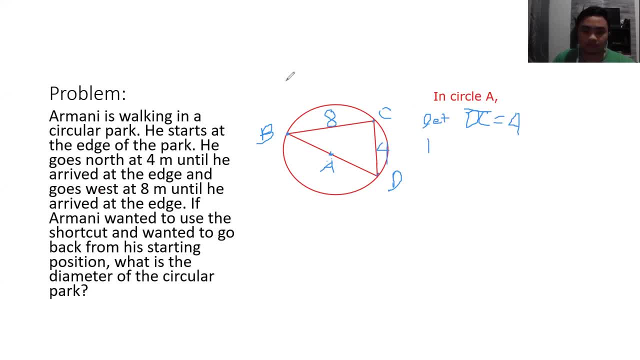 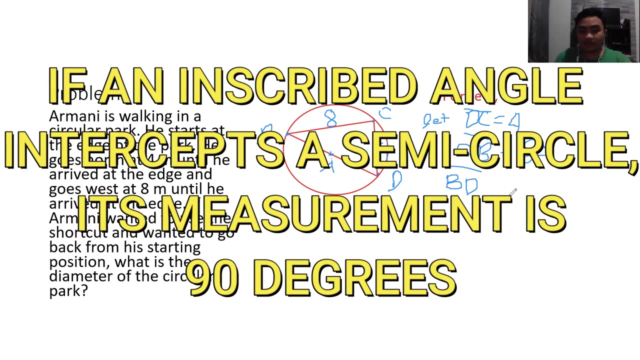 And let, Sorry about that- And let CB Line segment CB equal to 8. What is line segment BD? So with that, With that problem, we are using the semicircle theorem. Why? Semicircle theorem states that when an inscribed angle intercepts a semicircle, then it is a right angle. 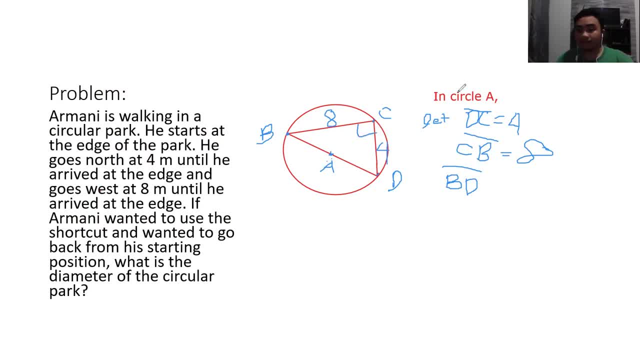 Therefore, this is the right angle, Why, Again, that is an inscribed angle right. It intercepts the semicircle, which is this right. So therefore the measurement of that is 90 degrees. So that is the semicircle. 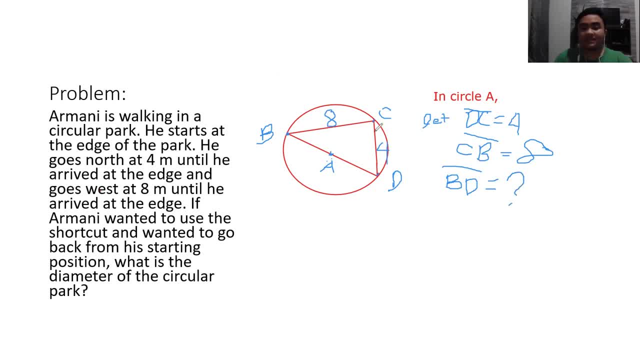 So find B With that. since this is 90 degrees, this would be automatically a right triangle. With that we could easily find the line segment BD through using the Pythagorean theorem. The formula for the Pythagorean theorem is: 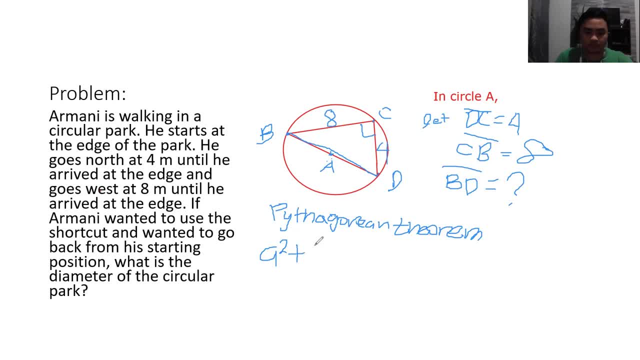 A squared plus B squared is equal to C squared, Where A and B are the sides of the triangle and C is the hypotenuse. Hypotenuse can be found opposite to the right angle. So let us now substitute our given. So we have first A, which is 4.. 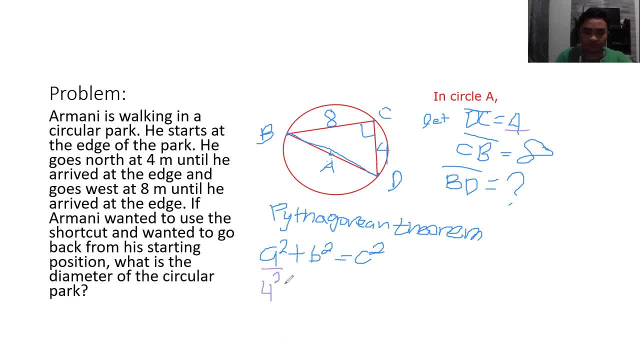 So we have 4 squared plus B, which is 8.. We have 8 squared here is equal to C squared. Simplify them. So what is 4 squared is 16.. What is 8 squared is 64 is equal to C squared. 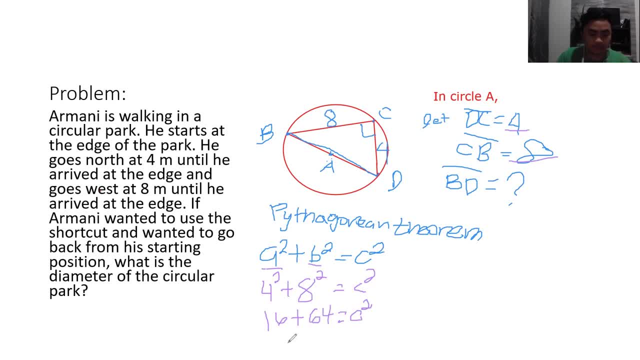 Simplify them So we have: 16 plus 64 is 80 equals to C squared. To get rid of the squared we need to square root them. So the square root of 80 is C is equal to 8.94 meters. 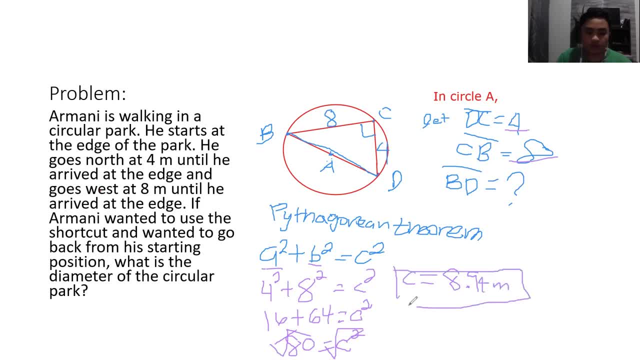 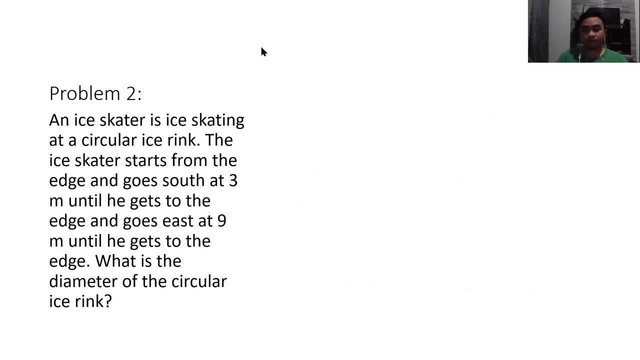 So, therefore, the diameter of the circular part is 8.94 meters. For this next problem, I want you to pause the video and try to answer it. Go, I think you are done answering, So I am going to answer. 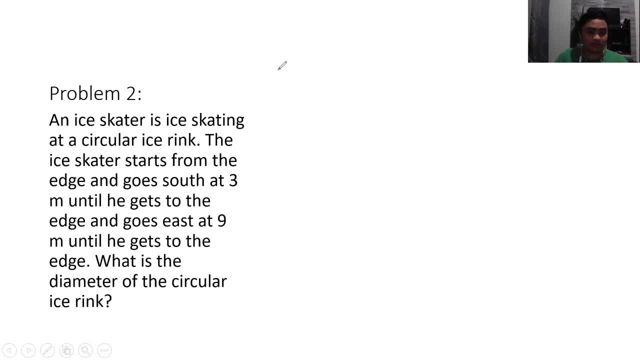 I need to review. So the first thing that we need to do is to visualize and illustrate the problem. So an ice skater is ice skating at the circular ice rink. The ice skater starts from the edge and goes south at 3 meters until he gets to the edge. 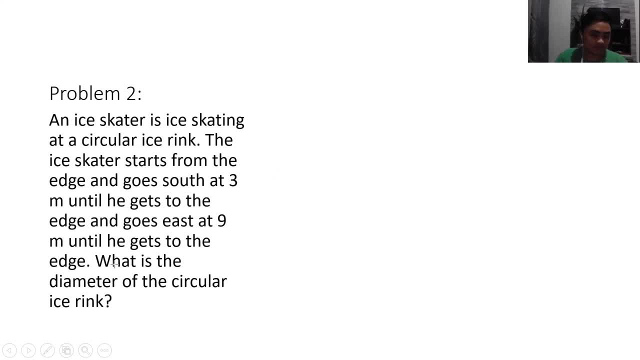 and goes east at 9 meters until he gets to the edge. What is the diameter of the circular ice rink? So let us first draw a circle, Since it says here the ice skater starts from the edge and goes south at 3 meters. 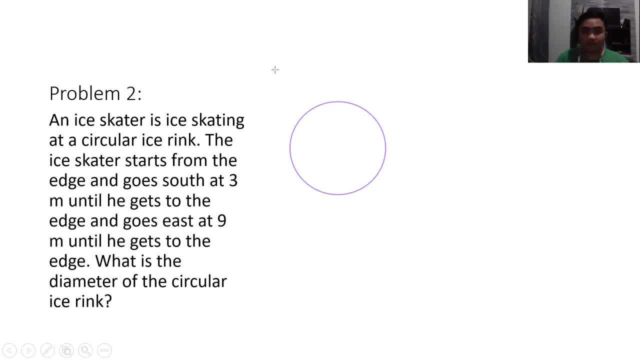 until he gets to the edge and goes east. So probably our starting point is here And he goes there. That is it. The next instruction is: The ice skater starts from the edge and goes south at 3 meters. The ice skater goes east at 9 meters. 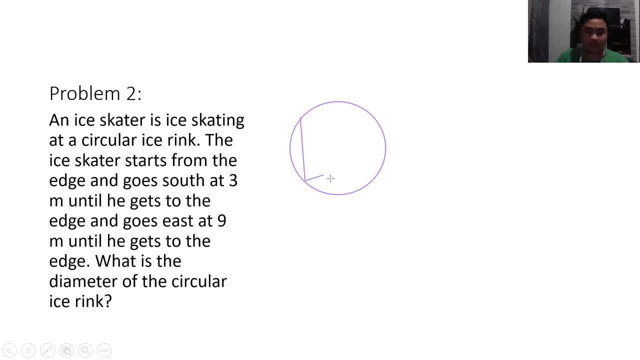 So let us go east until he gets to the edge. So let us go here. So what is the diameter of the circular ice rink? So this is the diameter. Through the semicircle theorem, this angle would be 90 degrees. 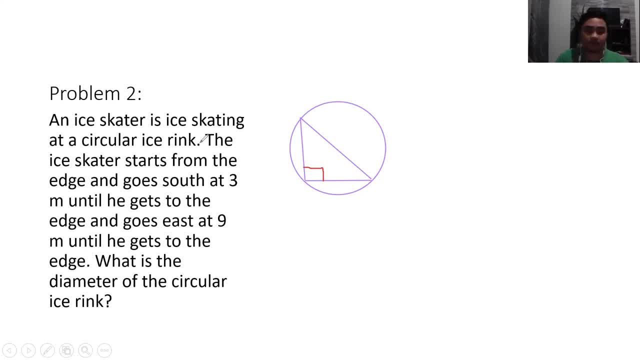 And this would be a right triangle. The first is It goes south at 3 meters, So let us identify this as 3 meters, And it goes east at 9 meters, So let us say that this is 9 meters. 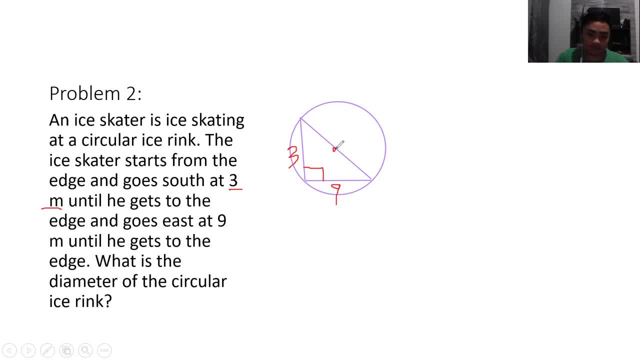 So let us use math. So this is point M, This is point A, This is point B And this is point H. So let us start. So, in circle M, let line segment HT be equal to 3.. 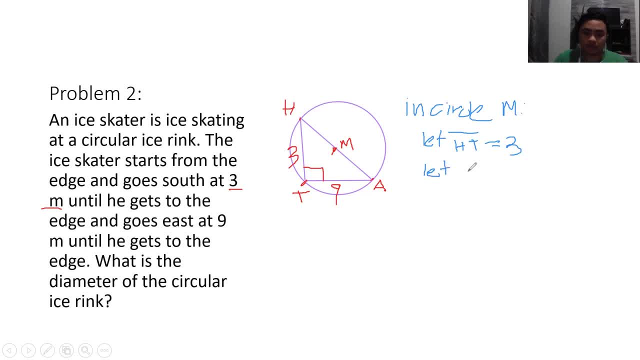 And let TA Line segment TA be equal to 9. Find line segment 8H. So that is the question. With that we could use the Pythagorean theorem in order for us to find HA or line segment HA. 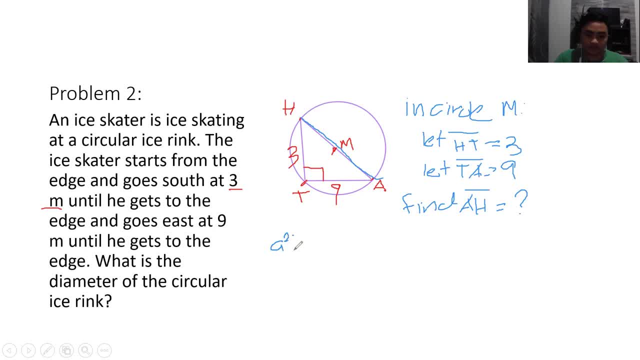 So formula again is: A squared plus B squared is equal to C squared, So A is 3.. So I have 3, squared plus B is 9.. So I have 9. squared is equal to C squared. Simplify them. 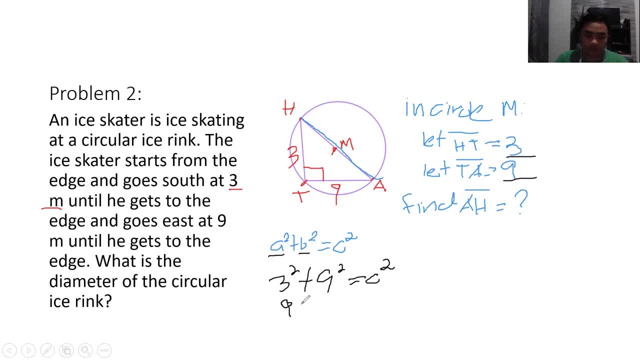 So what is 3 squared is 9.. What is 9 squared is 81 is equal to C squared. Simplify them. So we have 9 plus 81. We have 90 is equal to C squared. To get rid of the exponent 2, we need to square it then. 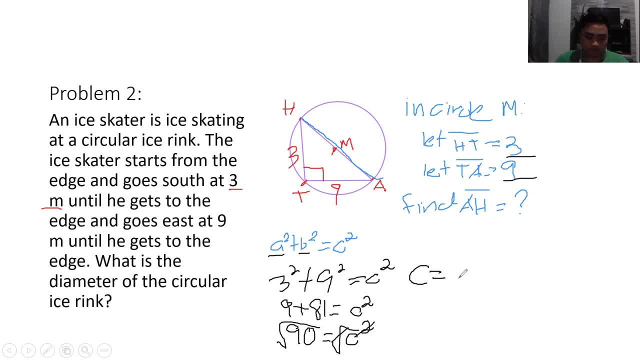 So C now is equal to 9.. So we have 9.49 meters. So therefore the diameter of the circular ice ring is 9.49 meters. That's it.